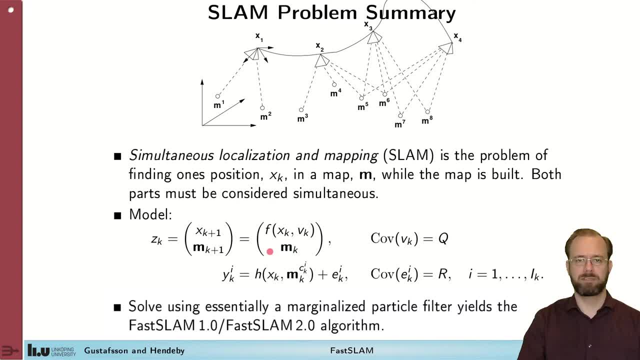 before and a map that is static in time, So there's no process noise changing this over time. We make observations of landmarks that we're stacking in the map and the measurement equation relates these landmarks to the pose of the sensor. We don't know in a general setting from what landmark a specific measurement 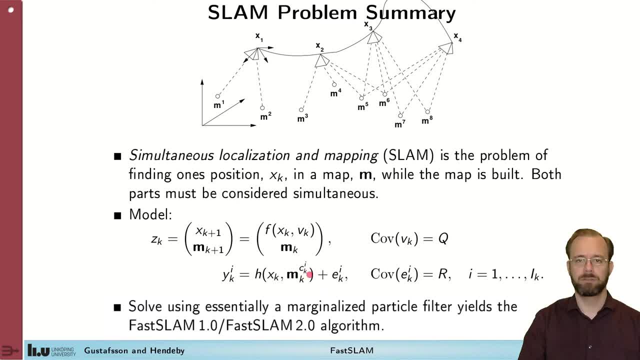 comes. so we need to do an association, And the association here is denoted by this CKi, which says that at time k, the i-th measurement relates to the position of the sensor. So this is the position of the sensor that relates to this specific landmark. 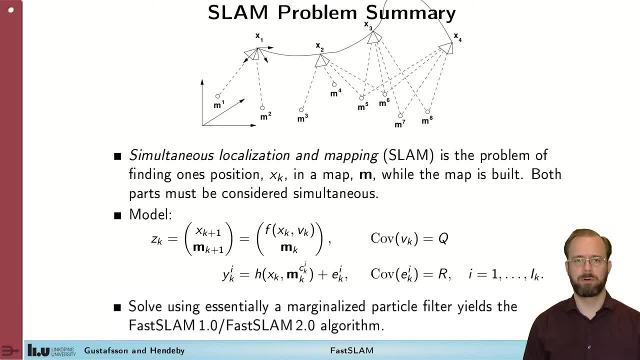 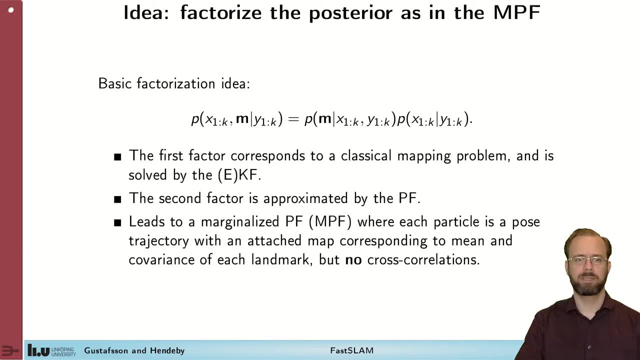 In this video, we'll solve this problem specified by this model using FAS-SLAM, which is a marginalized particle filter. Just as in the case of the marginalized particle filter, the key component to solve the problem is to factorize the posterior direction. 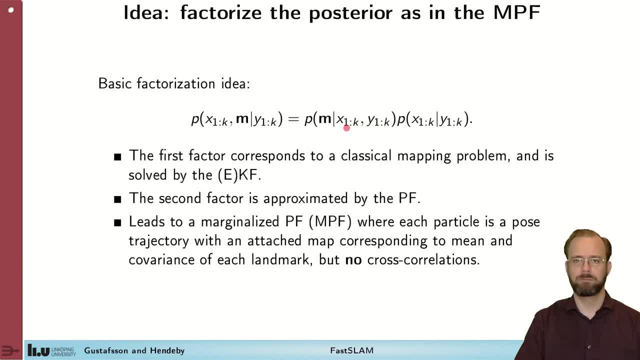 If we look at the posterior distribution here. so it's the full trajectory of the sensor platform and the map given the measurements. it factorizes in two parts: One is the determination of the map, given the trajectory and the measurements, and the second part, that is, finding the trajectory. 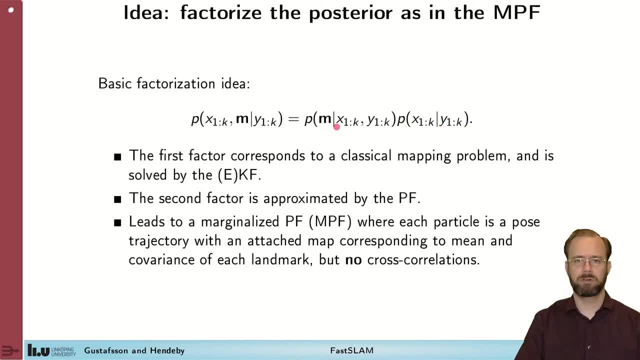 given the measurements, The first part here is treated using a Kalman filter- extended Kalman filter- depending on the non-linearities in the measurement equation- whereas the second part can be treated as a particle filter, And this is exactly what we do with the marginalized particle filter. 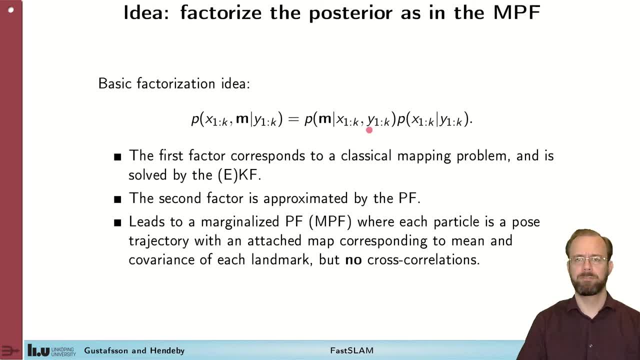 One important property that we receive by making this factorization here is that the first term that relates to the map is the final value of the parameter, and that is defined by the linearity of the parameter. That means that the corresponding data is generated by the linearity of the parameter. 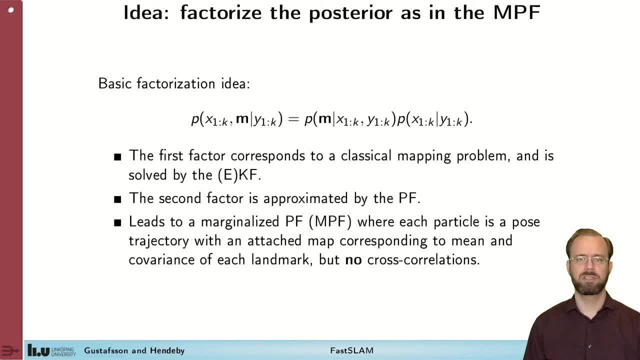 and the linearity of the parameter is the linearity of the vector and the linearity of the vector And we can treat all the landmarks individually. It gives us a complexity benefit compared to the extended Kalman filter where we need to treat them all at the same time and the cross correlations between them are important. 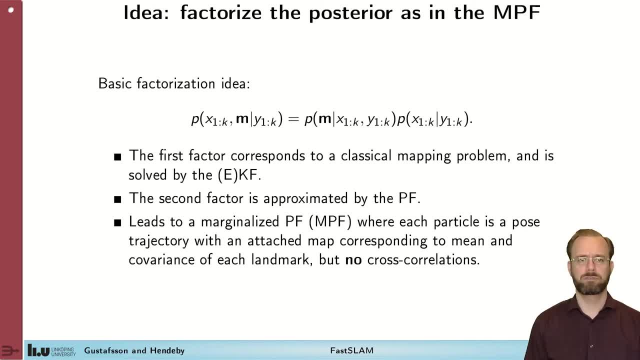 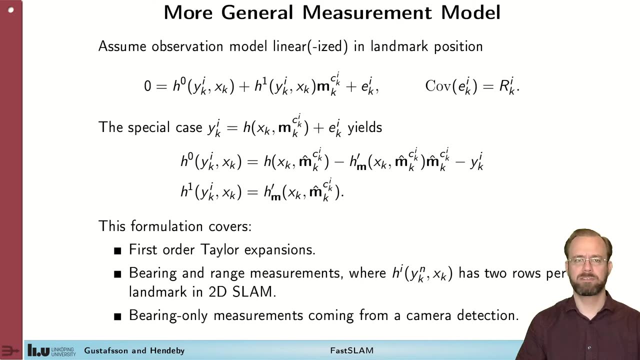 How can we just lose the cross correlations? Well, we don't. They are encoded in the particles instead. So we need to use particles that encode that information. information is: Before I can go on and outline the PASS-SLAM algorithm, I'll have to reformulate. 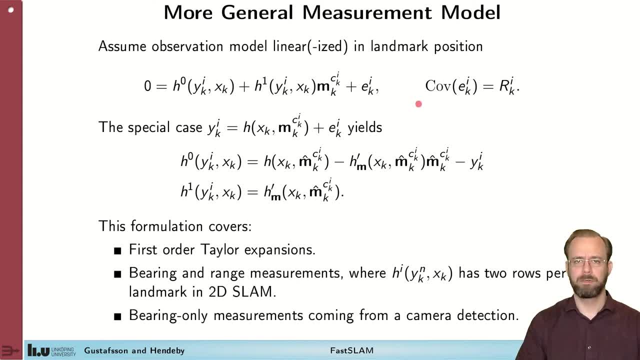 the measurement equation on this form. I do it because we need to highlight the conditional linear behavior in terms of the map which is necessary for the marginalized particle filter to work out, and because this is a form that is quite generally applicable For our normal measurement. H0 and H1 up here can be given by these expressions here. so 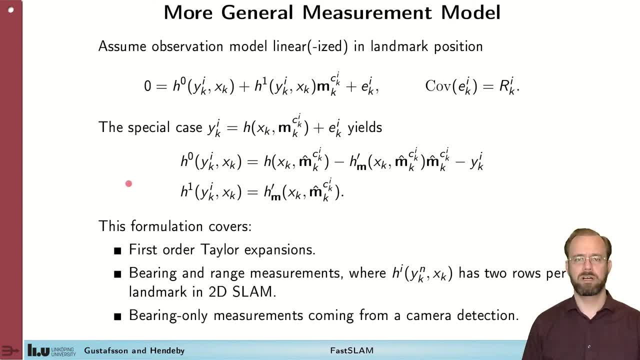 they fit. The formulation that I've used here covers first-order Taylor expansions of most common measurement equations. It fits well with the bearing and range measurements and where we have two rows per landmark, and it fits well with bearing-only measurements coming from a camera detection, for example. So it's applicable to all the sensors that. 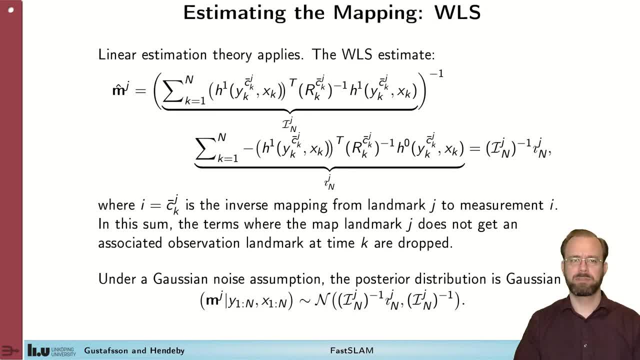 we consider As a first step in outlining the PASS-SLAM algorithm, we'll look at how to estimate the map And, as I said, the map components, the landmarks, are independent, so we can estimate them one at a time. So we'll start by looking at how to estimate. 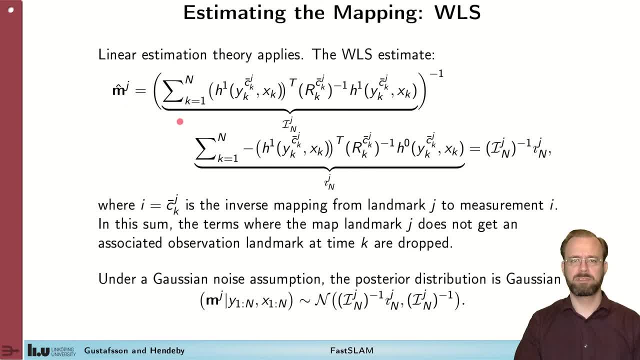 the map. So we'll start by looking at landmark J. given all the measurements that we have received of landmark J from time, k equals 1 to n. This is a linear problem, a linear batch problem, which we can then solve with the weighted least squares. So if we insert the 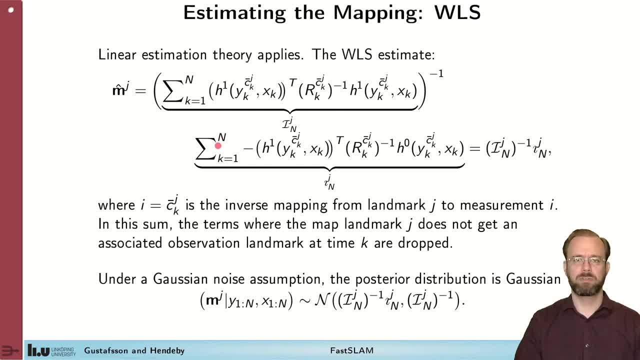 weighted least squares solution from previous videos to solve for the landmark J. here we get these expressions. They look more pricey than they do, but they're not. So we'll start by looking at how to estimate the map components, these landmarks. It's usually definitely more pricey than they are. it's more or less putting in the 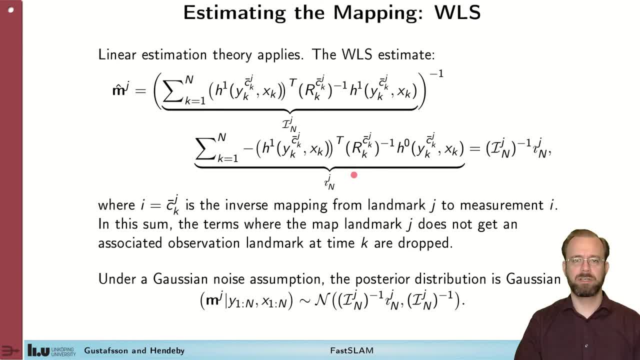 information that we have. What's been introduced here is C bar, sub k, which is the mapping from landmark J to the measurement I. that was used at time k for this landmark And we need some association for that, but we don't consider how to do that. 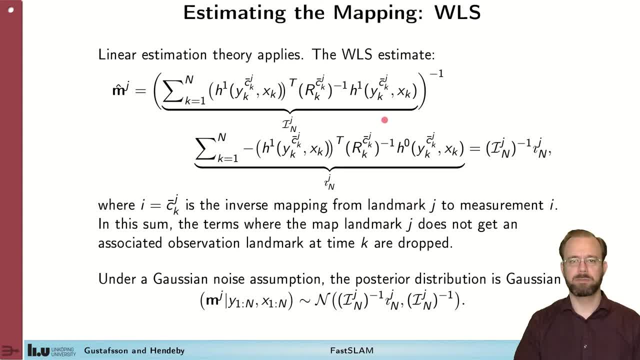 Also for the future we will map them based on randomness, But for the later projects we can use one metric system essentially To organize these. else, denote this thing here, that we take the inverse of capital I, which is the information for this landmark J, and we have the second part here, which is the 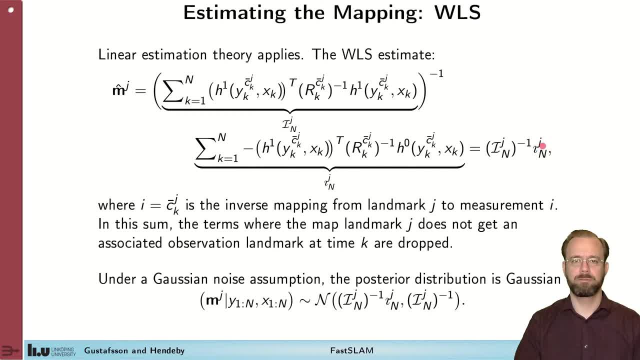 information state for the landmark J. We should also observe that under Gaussian noise assumptions etc. we can give a posterior distribution for the landmark. given the measurements and the trajectory, It's a Gaussian distribution. that's well. this mean that we compute from the way to least squares and the 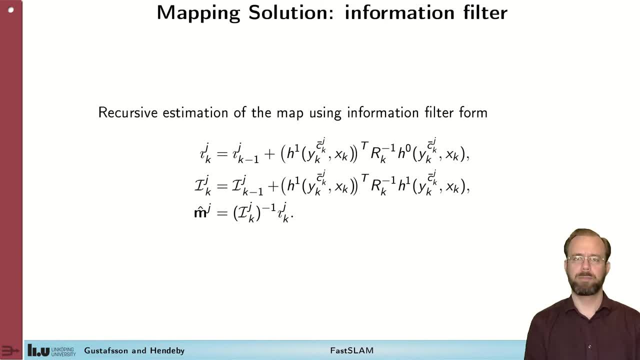 inverse of the information for covariance, We want to compute the map recursively, which we can do with information filter. You see the equations here. it's basically take the way to least squares solution and just adding one term at the time to this information, information state and we can from that extract the. 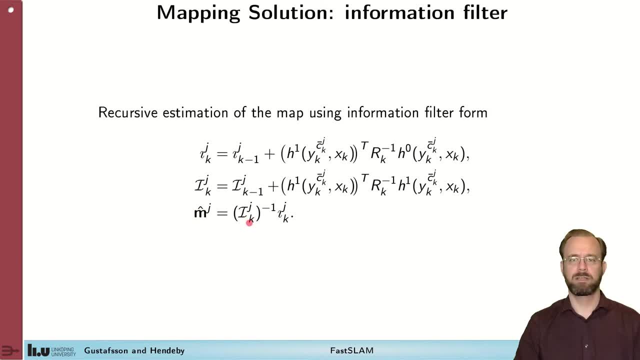 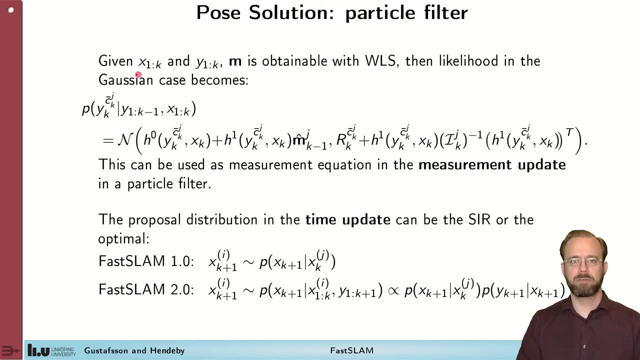 landmark position by multiplying the information state with inverse information. We will now show how we can solve for the pose, the trajectory, using a particle filter. One of the first things that we need to do is to solve for the position of the landmark. The most important part of this derivation is the fact that, given the 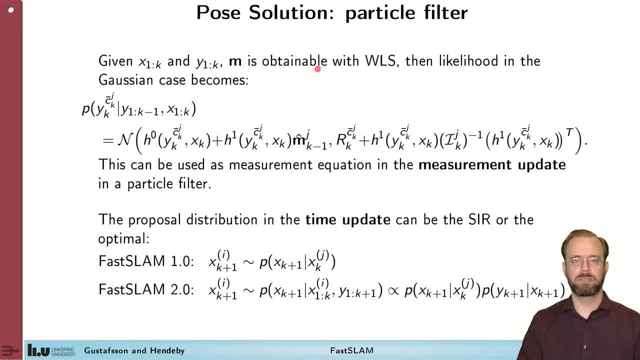 trajectory and the measurements. the map can be solved for using an ordinary way to least squares solution, as we've just seen, And we were also able to derive a expression for the uncertainty of the single landmarks. That means that we can construct a measurement likelihood here for a specific measurement. 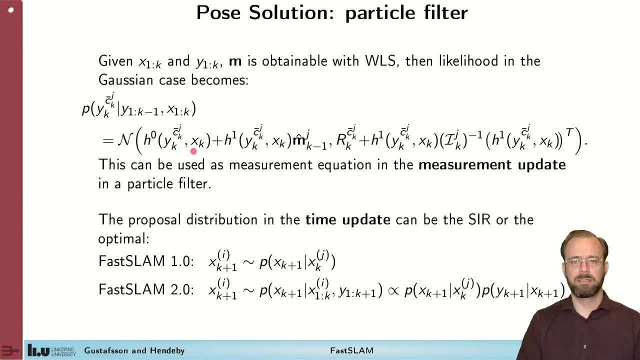 that match to a certain landmark. that is based on the measurement equation. combined with the uncertainty in the map as extra measurement noise, This can be used as normal measurement updates in the particle filter to weight the particle weights, The next part that is needed in a particle filter. to conclude, 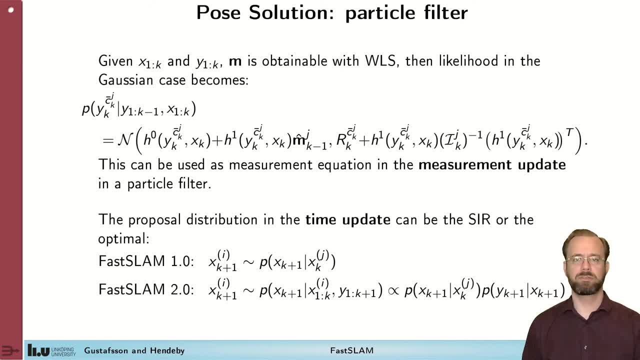 this PAS-SLAM algorithm is how to time update the pose. There is two different methods to do this. The first one, suggested, also denoted PAS-SLAM 1.0, is to use the same method as in the SRI particle filter. 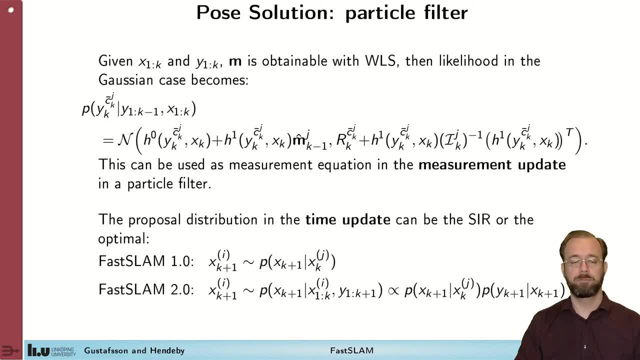 In an, In an update to FASLAM 1.0, FASLAM 2.0, it was instead suggested to use the optimal proposal, which includes also the measurements here, and we can see that it's partly the same prior. 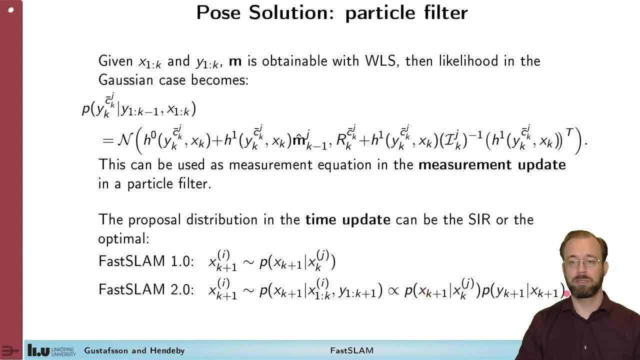 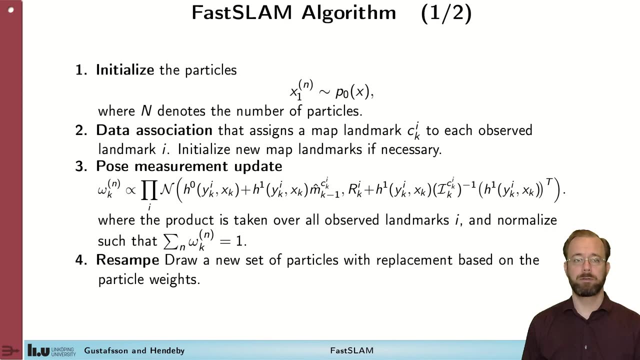 as in FASLAM 1.0, but also including the measurement likelihood. This makes the particle counts better, so we get particles in a better place, so we need fewer particles. So we are now ready to summarize the FASLAM algorithm. 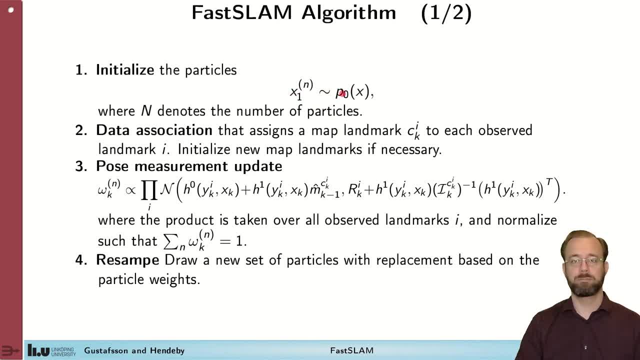 We start by initializing particles. according to some information about the pose of the essential platform, We perform data association. Note that this is done per particle in this case, so it's not as essential to get it right as in the extended Kalman filter SLAM solution. 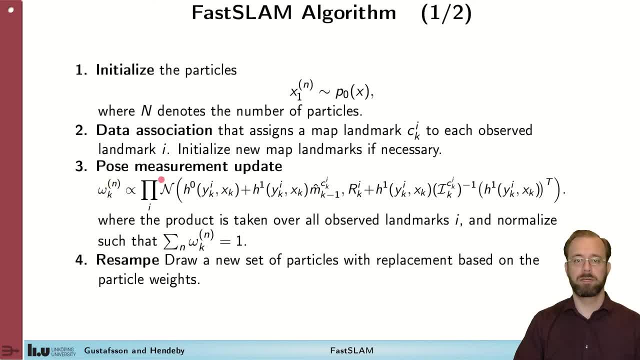 We update the particle weights using this equation here. that's based on this measurement equation listed on the previous slide. Afterwards, of course, we need to normalize the weights. Resampling can be performed if necessary, and in this case, we also resample the maps. 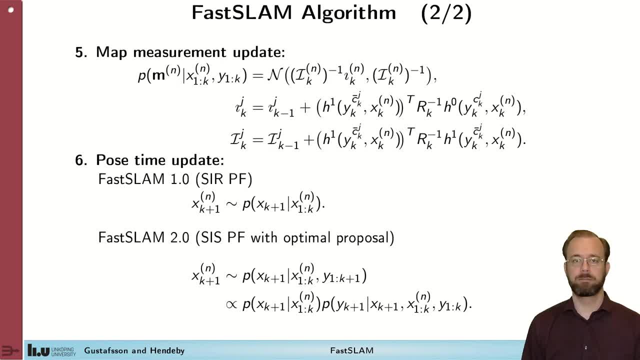 so the maps match the particles. Next, we need to do a measurement update of the map. So we use the pose and the measurement to compute the map using the information filter And then we make a time update in the particles based on either the SIR-R PF proposal or the 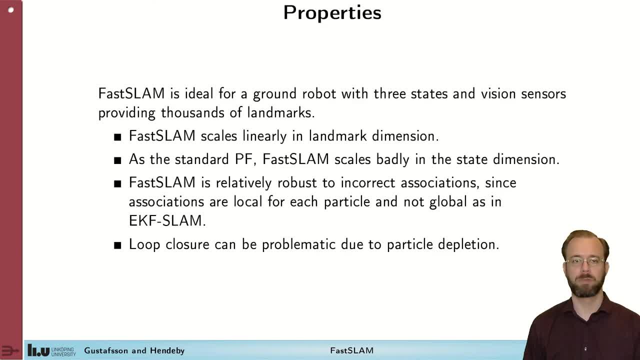 optimal proposal in the FASLAM 2.0. That is the FASLAM algorithm. Here are some of the properties that I would like to highlight. It's actually a really ideal method for ground-moving vehicles with a small state space and vision. 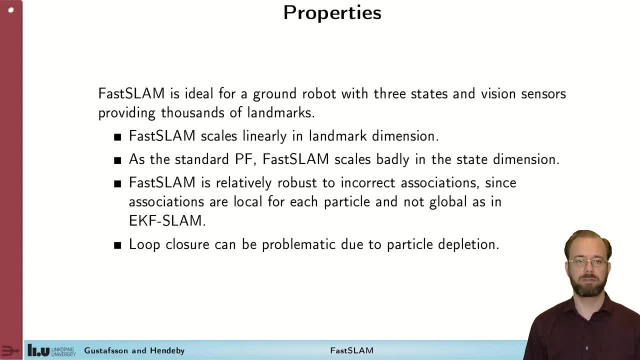 sensors. that provides a large amount of landmarks because it treats the map in a good way for that, And the reason for this is that it scales well with the landmarks. It scales linearly, At least in theory. You might need more particles to do that. 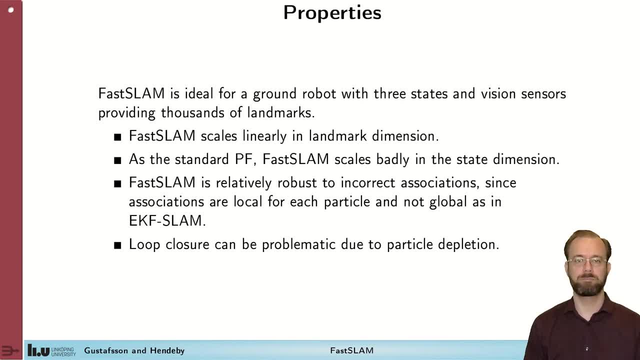 But it's a good way to do that. Next, we need to do a measurement update. Actually, there's no real data that covers the correlations, but in theory it's linear in the landmarks. But as the standard particle filter it handles large state dimensions, so-so 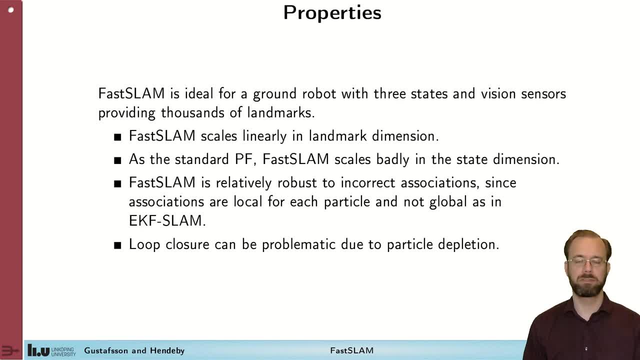 So if we would have a large state dimension of six or more, maybe that would be difficult to solve with a particle filter. but for small state spaces, as suggested here with the ground-moving vehicle with three states, it's ideal. It's also more robust towards association errors, which is nice, since we make the associations. 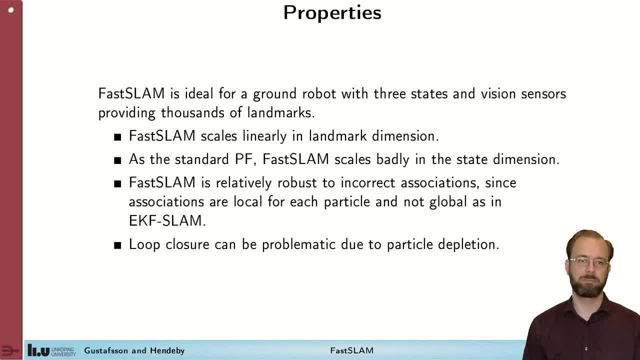 per particle instead of globally, as in extended Kalman filter SLAM, for example. we get the diversity in different associations and overall we would probably get a good solution. Closure is poorly handled in the particle filter SLAM. here That's because we get particle depletion in the past and hence when we see a landmark 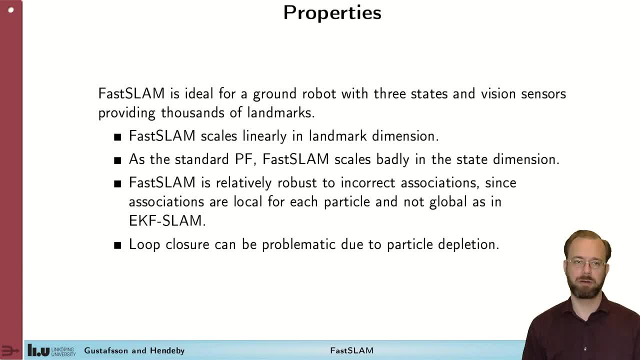 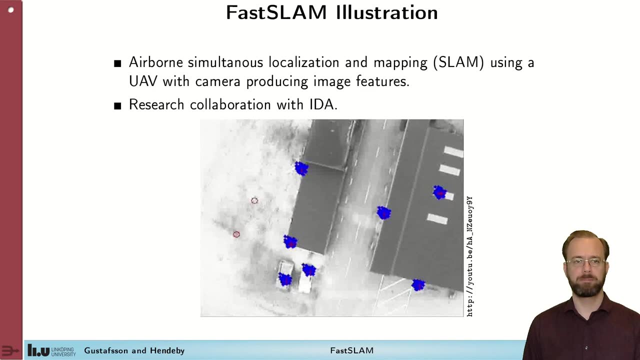 that we haven't seen for quite a while. there's little diversity in the particles to actually make any changes. In that case, the extended Kalman filter SLAM is much better. I'll finish with an illustration Illustration of fast SLAM before we conclude this video. 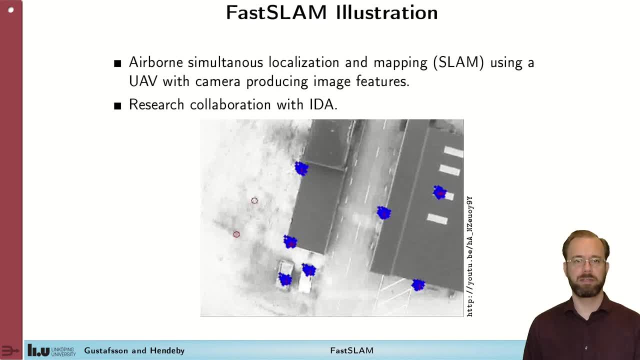 It's an example of a project that was jointly run by Atmatic Control and IDA. It's an airborne UAV looking down using a camera where we, in this case, use fast SLAM for positioning. We will see landmarks with red dots and blue particles representing the map. 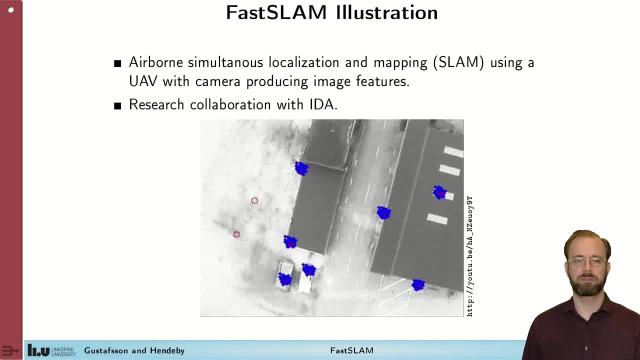 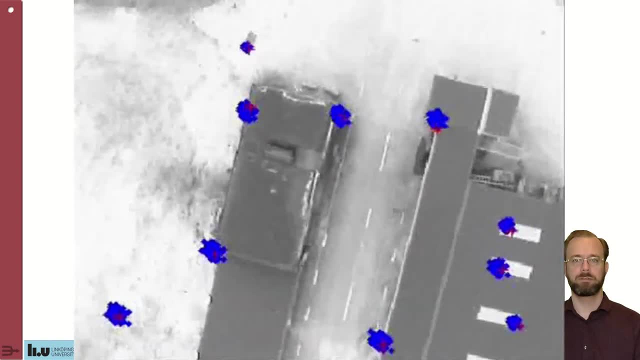 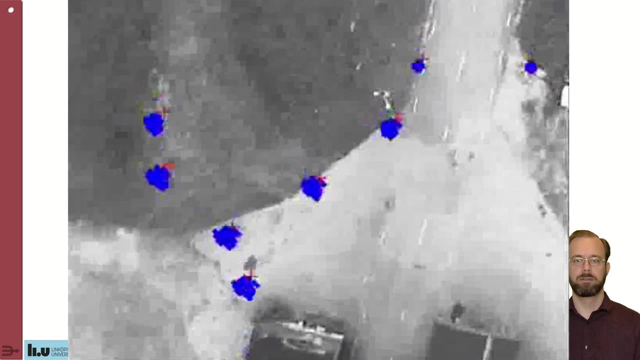 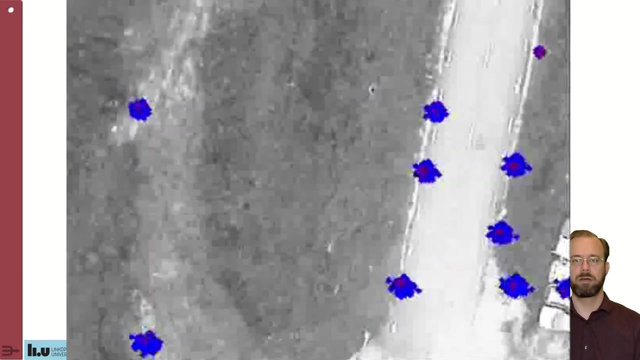 We're going to fly over this and you'll see how it progresses over time And you can see how the clouds of particles around the red landmarks grows as we see them more and how it fairly well follows the appropriate position on the ground with the landmarks. 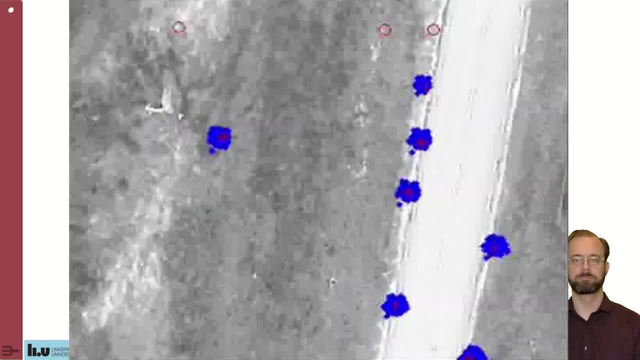 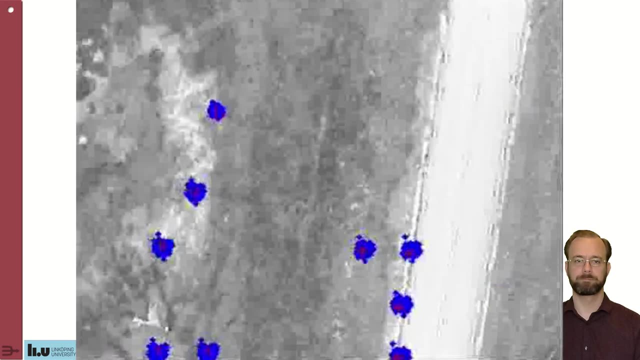 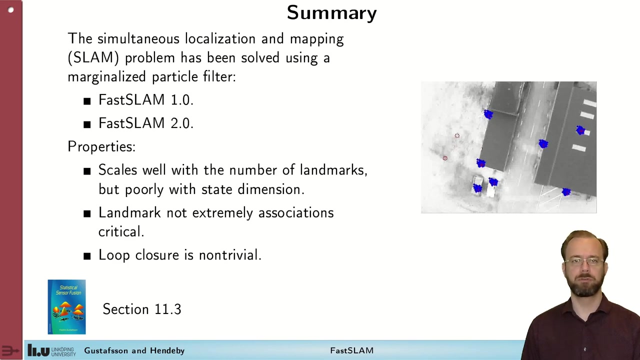 indicating that the map and the positioning is working well. Thank you. We have no closure in this case, so we don't see the problem of that. So, to summarize what we've done in this module, we have looked at the simultaneous localization and mapping SLAM problem and it has been solved using a marginalized particle filter. 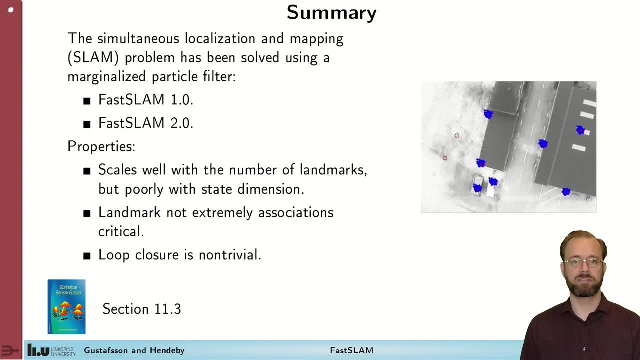 This resulted in two methods called the fast SLAM 1.0 and the fast SLAM 2.0. They are quite popular in literature, especially for ground-moving robotic vehicles with lots of landmark measurements but a small state space. Important properties to highlight is that the methods scale well with the number of 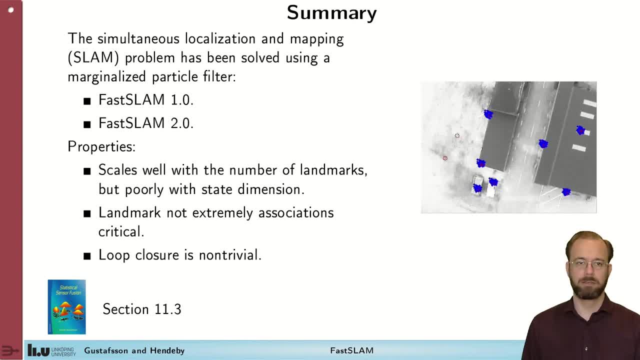 landmarks, but poorly with the state dimension. That also explains why it's popular in the robotics community. Landmark associations are not extremely important. They are not necessarily the most important. They are not necessarily the most important. They are not necessarily the most important. 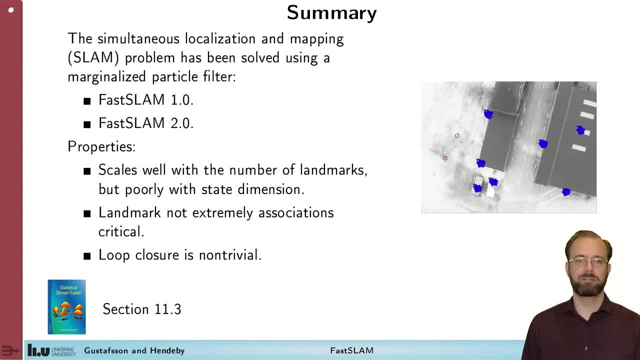 Unfortunately, fast SLAM handles load closures poorly, but there are methods to get around that if necessary. To read more about fast SLAM methods, look in the textbook in section 11.3..